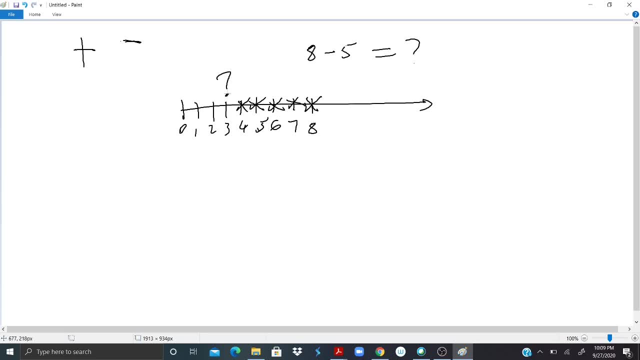 So what is this number right here? From the eight I subtract five. So I will start counting from here to here. I'll have zero one two three. So the result here is three. I can also use counting the stone as we did previously. So I will be having one two three four five six seven 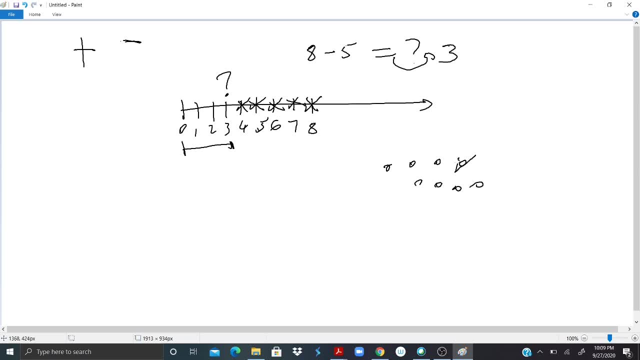 eight stone. If I subtract five like one two three four five. So how many stone left? I have one two three. So I have the same result three as here. Another example nine minus four. This is equal to five. So from our number line one two three four five six seven 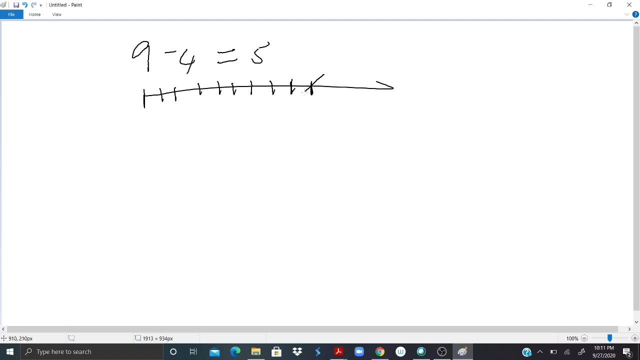 eight and nine we will be subtracting four. So one two three four. So what is this number? Let's count. 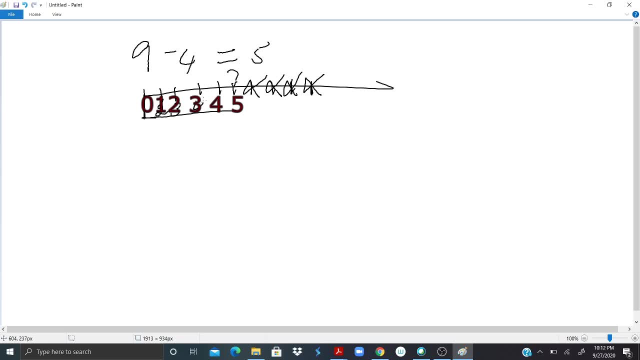 Give me one two three four five. So same as we found here. So before we continue find this by 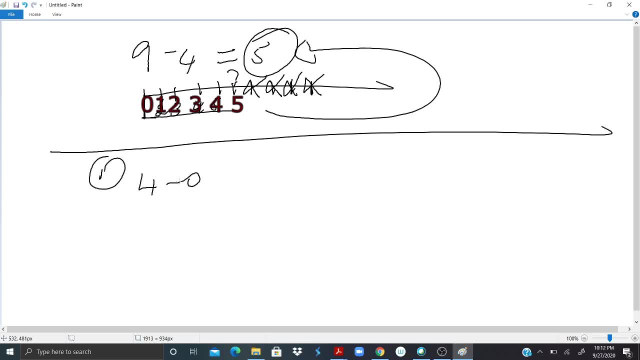 yourself. First four minus zero. Second eight minus five. Third ten minus three minus two. Put 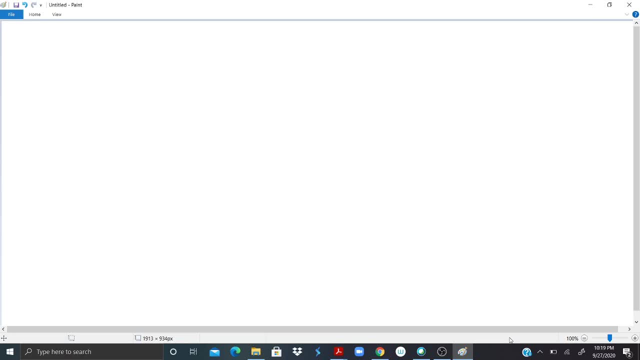 your answer is that in the comment section. So now moving to multi digits we line them up the same way as we did for addition. But in this case make sure that the order is respected. If I say for instance 25 minus 12 you should write 25 first and then minus 12. This is the right way. You don't write 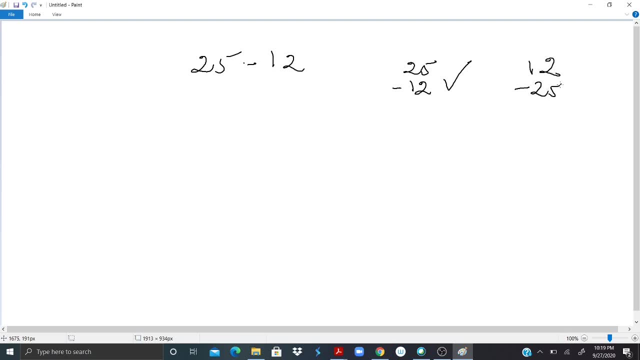 12 minus 25 then you modify the place. This is wrong. So what you should write is 25 first on top and the 12 at the bottom and from here you can proceed to the 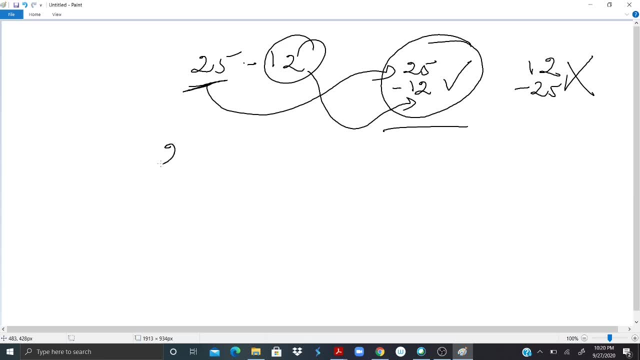 operations so as we did for addition 25 minus 12 right we will proceed from the right mouse to the left but before we do that let's talk about something we call 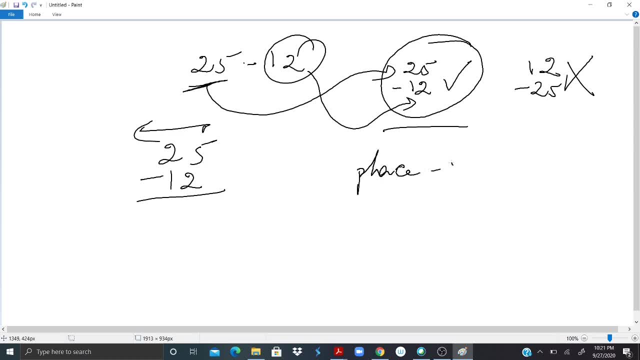 place value place value if I write one it is only one digit and it's one place that I use if I write like for instance 32 in this case I use two places the first place is 42 and the second place is 43 if I write 149 yeah I'm using three places 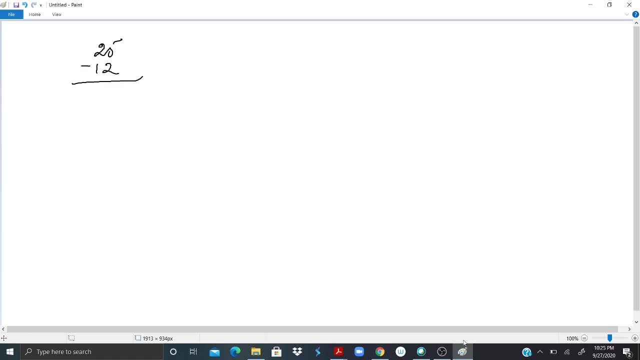 two three so back to our subtraction 25 minus 12 I will do 5 minus 2 I will have 3 I will do 2 minus 1 I will have 1 so 5 minus 2 3 2 minus 1 1 good for that 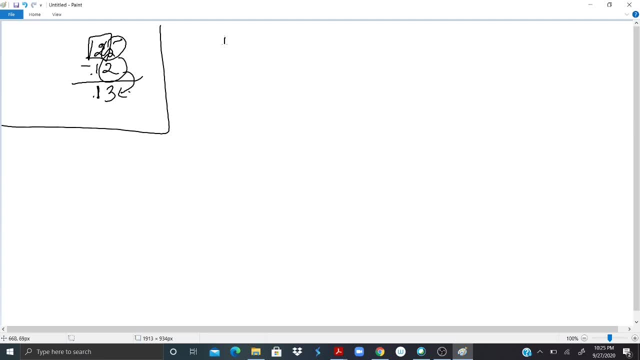 another example let's do 1 23 minus 5 2 times about 1 2 times into 1 minus 5 one 1 23 minus 5 okay let's start so 3 minus 5 right okay there is a problem because 3 is less than 5 I can now subtract 5 from 3 so what I do is I look at the next place is there a number there yes then I will borrow 110 from the next place so I'll borrow 110 from the next place so I'll go from the two tens and i will add it to the three and we will make the three thirteen so supposed to be 23 i borrowed one ten from the two second digit so here i'm left with one now i can subtract five from the thirteen so thirteen minus five eight here i have one left so i'm not using these two i'm using the one one minus 19 i have one one minus 19 i have one so my final answer is 1 18 let's do one more example 305 minus 47 so five is less than seven i will go to the next place to see if i can borrow but i see zero over there i cannot borrow from zero so i 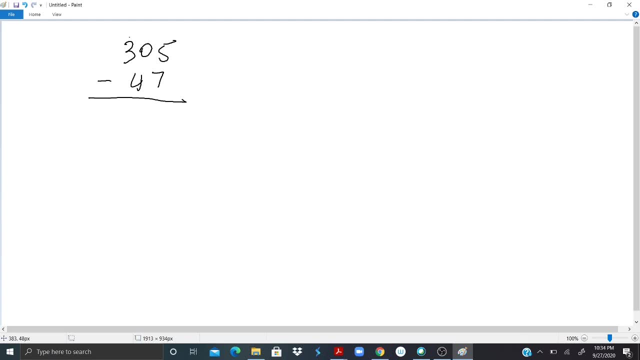 look to the following place to see if i can borrow i see three okay so that means i have three hundreds and i will borrow one hundred so once i borrow 100 i will split it into nine tens and ten ones so the nine tens i will put it right here and the ten ones i will add the five and this will give me 15 now i can perform my operation 15 15 minus seven have eight i move here i'm not using the zero i'm using the nine nine minus four that's five and here since i borrow the hundred this one becomes two so i'm not using the three five 2 minus nothing is 2. So, my final answer is 258. Let me redo it here. 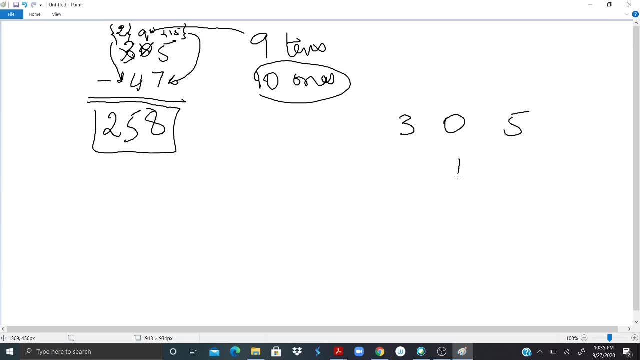 3, 4, 5, 4, 7. Right? 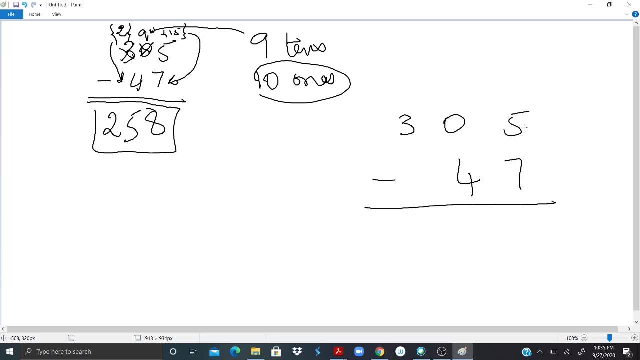 Minus. I want to subtract 7 from 5. I realize that 7 is greater than 5. I have to look to the next place to see if I can borrow 1 tenth. Unfortunately, I see 0. So, I move to the next place which is the 100th place to see if I can borrow. 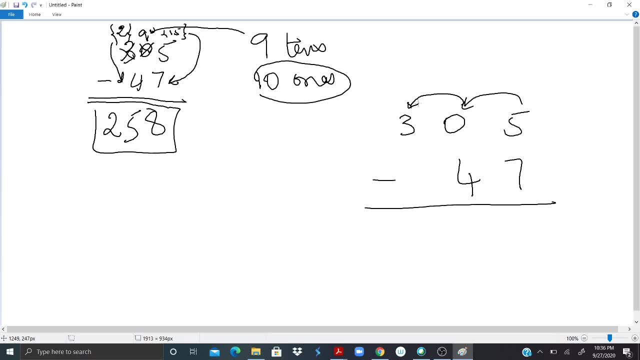 Yes, I can borrow 1 hundredth. So, I borrow it. So, here I'm left with 2. So, from the 100 that I borrow, I will split it into 9 tenths and 10 ones. If I combine these, I should have 100. So, once I split it, I put the 10th value on top of the 10th place which is 9. And I put the 10 that I borrow here, I add it to the 5 and I put the result here, 15. Now, I'm not considering this line anymore. I'm using the top line here. 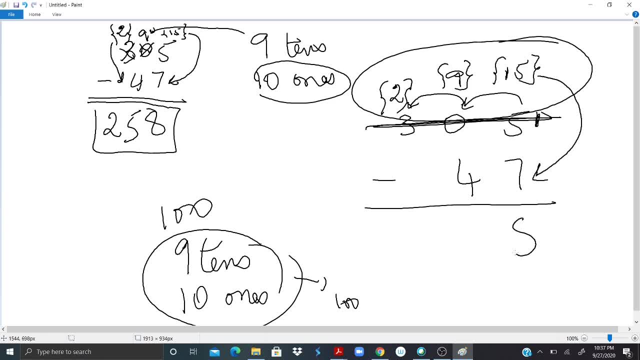 I will do 15 minus 7. That will give me 8. I will do 9. I will do 9 minus 4. That will give me 5. 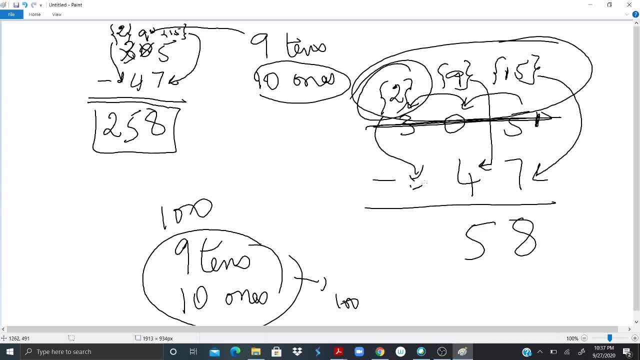 And I will do 2 minus 19, which is invisible 0, and that will give me 2, which is my final answer. 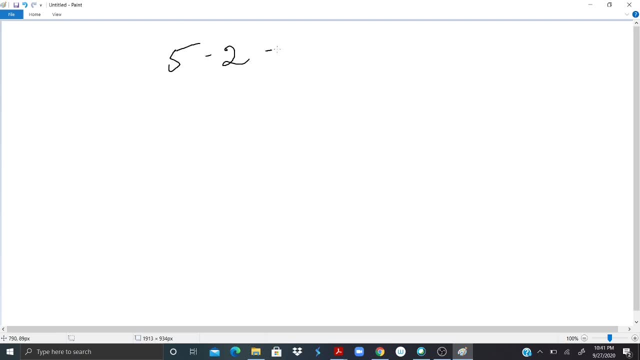 Now, suppose that I solve 5 minus 2 and I have 3 as a result. I did it mentally and I didn't use any number line. I didn't count anything precisely. But I wonder if I got it right. So, I wonder if I got it right. 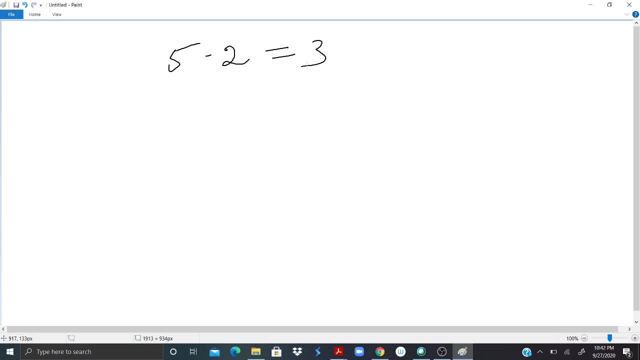 I want to prove my, I want to check my result. So, what to do is to take the result that you got, add it to the number you subtracted. And if you get the number, original number you are subtracting from, then that means your operation is correct. So, what I mean is I'm using 5 minus 2 and I'm getting 3. So, I will come back and say 3 plus 2. Is this giving me 5? Yeah. Is 5 the same right here? Yes. So, that means this operation is correct. 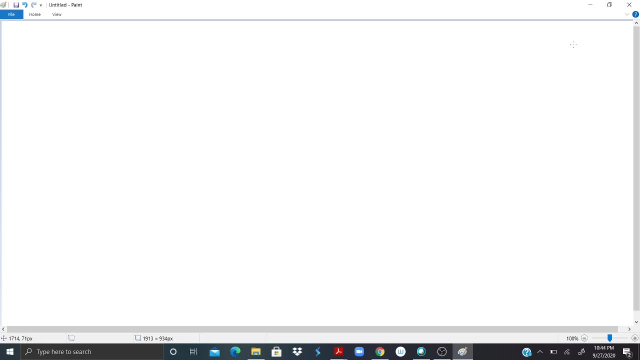 To finish this section, let's talk about properties when subtracting whole numbers. 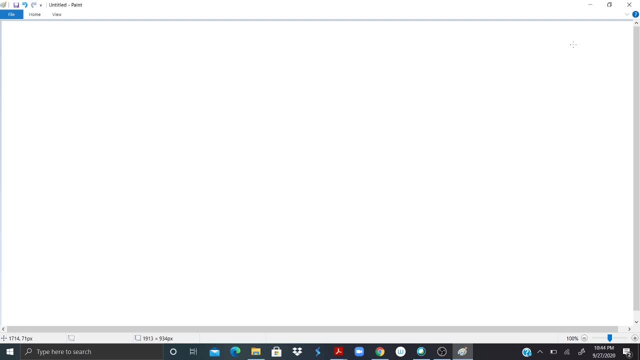 First, let's just say that subtraction is not commutative. So, we will talk about this one later. 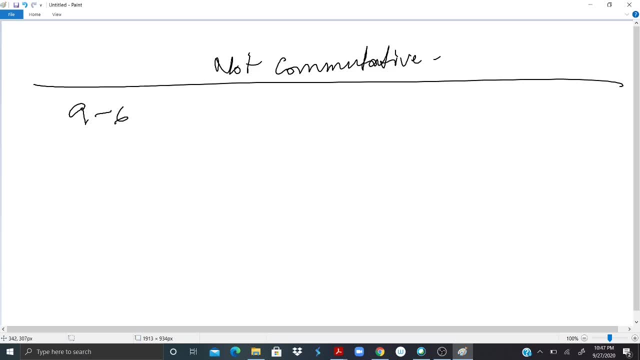 Second, let's do this. 9 minus 6 minus 1. So, next thing is to complete. 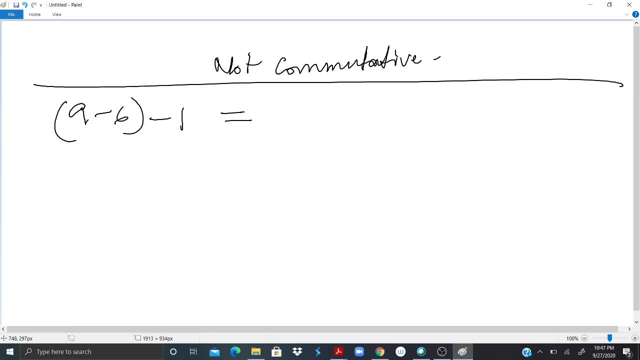 Complete what is inside the parentheses. And that will give me 3. 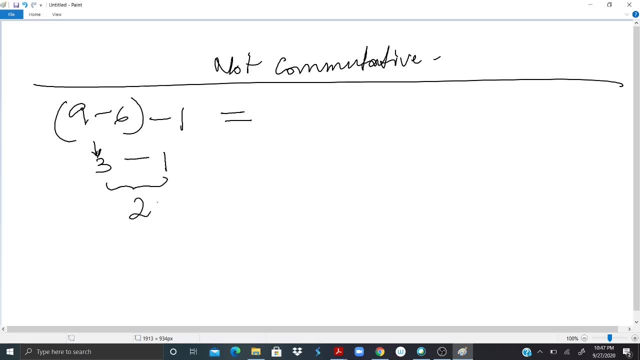 And 3 minus 1 will give me 2. So, my result here is 2. 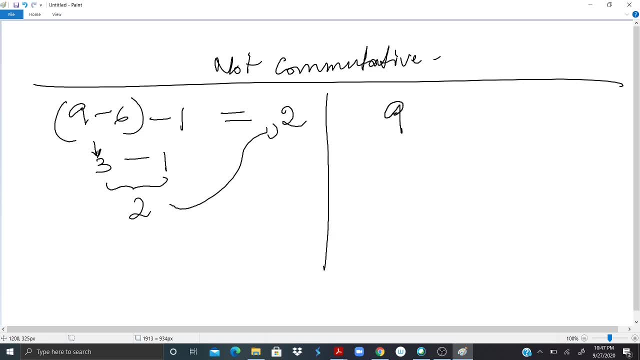 Let's just rewrite the same numbers. 9 minus 6 minus 1. And now, let's move the parentheses around the 6 and the 1. 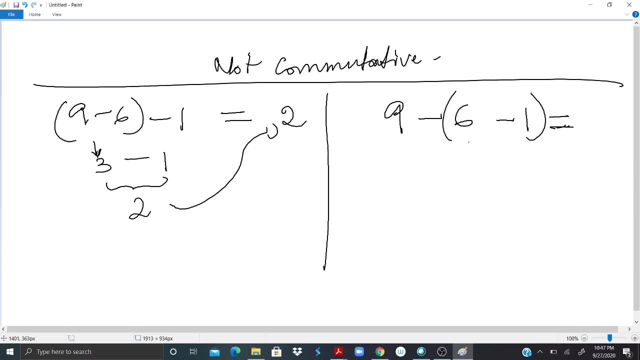 So, we will still do what is inside the parentheses first. And that will give me 5 here. 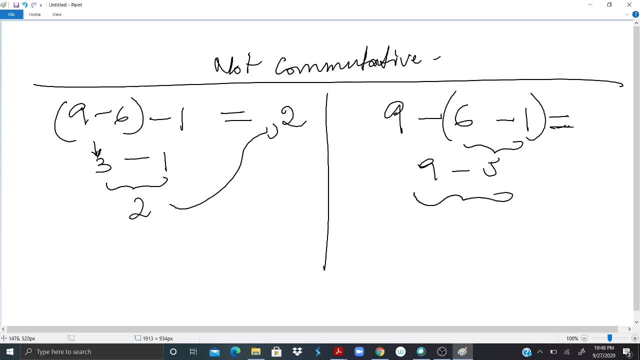 And I will do 9 minus 5. And my result will be 4.